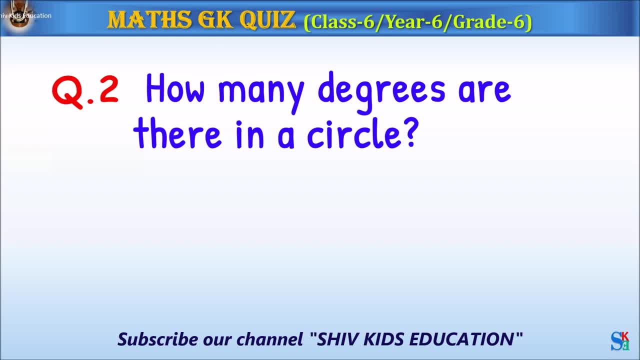 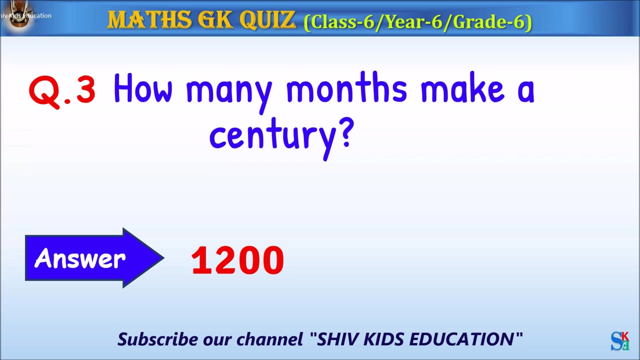 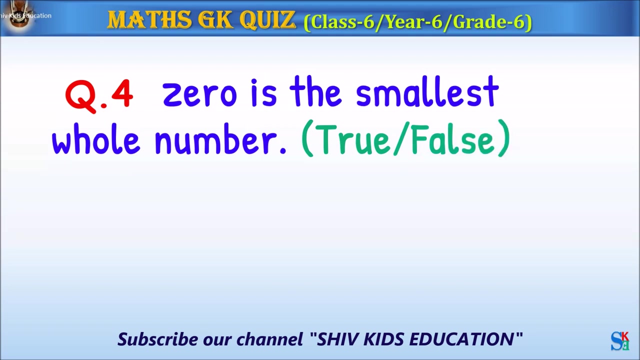 2. How many degrees are there in a circle? The answer is 360.. 3. How many months make a century? The answer is 1200.. 4. Zero is the smallest whole number. true or false? The answer is true. 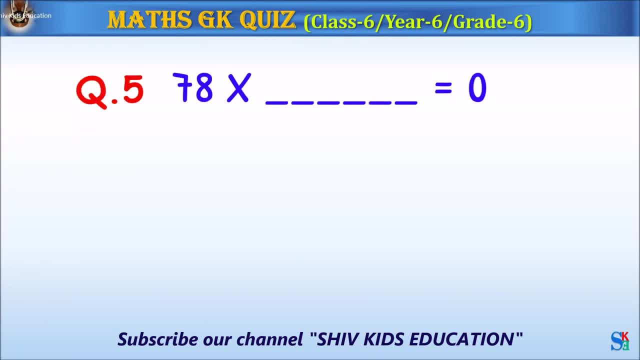 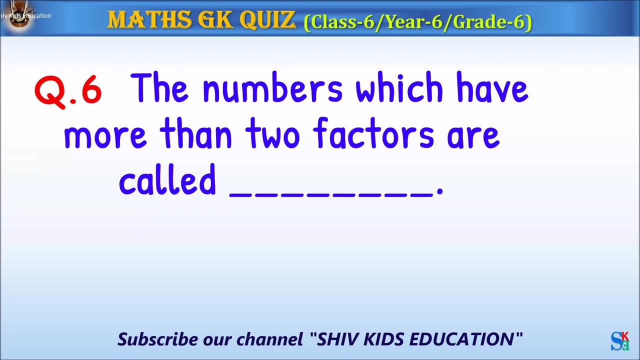 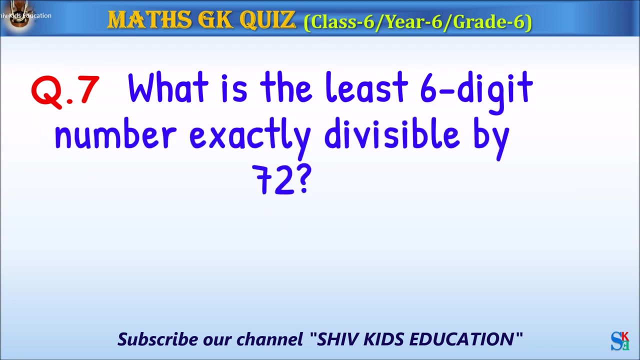 5. 78 times what equals zero? The answer is zero. 6. The numbers which have more than two factors are called what? The answer is composite numbers. 7. What is the least 6-digit number? The answer is exactly divisible by 72.. 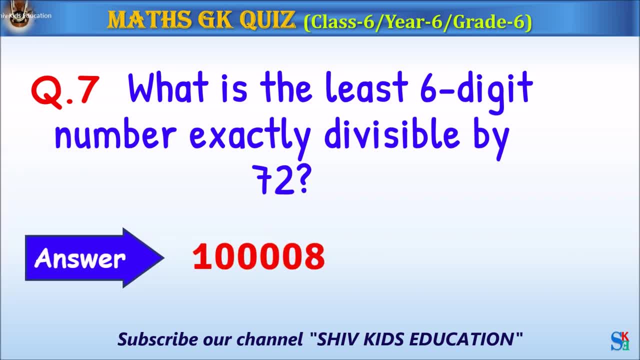 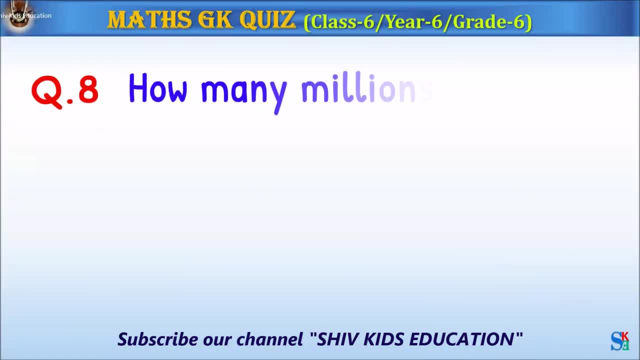 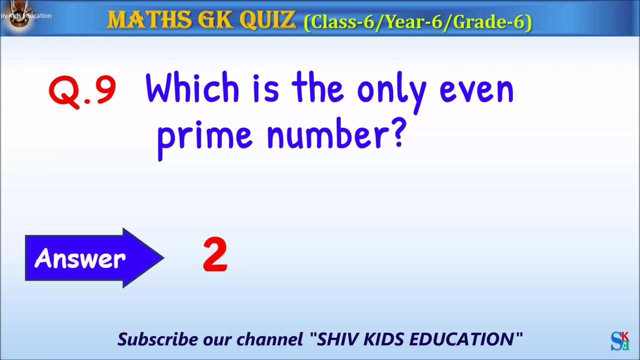 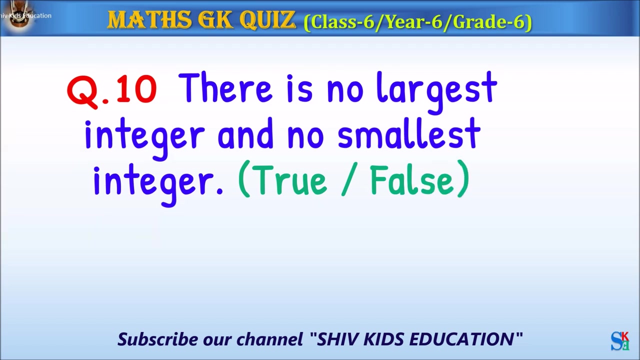 The answer is 100,008.. 8. How many millions make a billion? The answer is 1000.. 9. Which is the only even prime number? 7-divine Nervous definition n-tord. The answer is 5.. 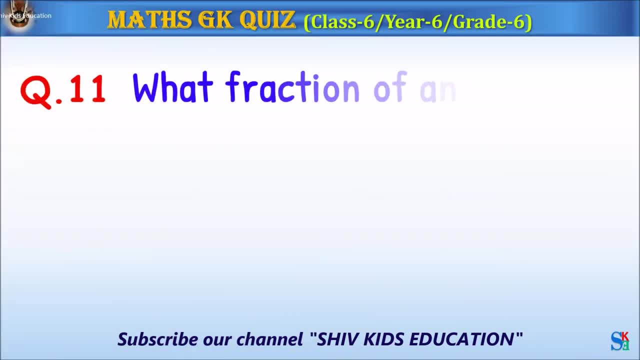 The answer is 4.. 5. What is the largest power, the smallest and the налignent factor of an hour? The answer is 2014.. 5. What is the largest of the elements? 12. 120 degrees is known as? what type of angle? 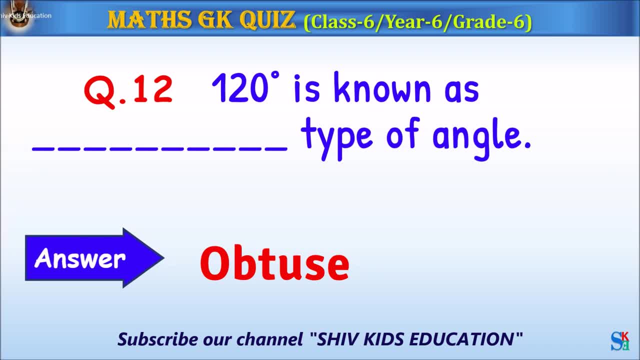 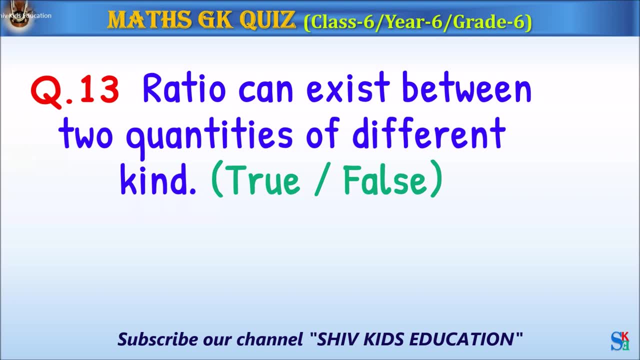 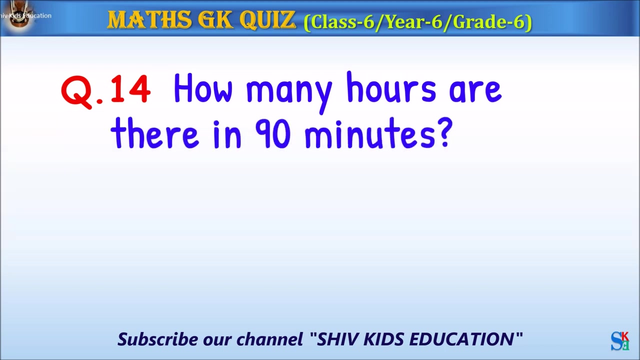 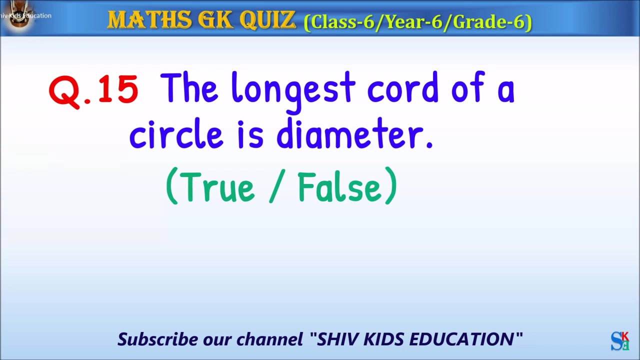 The answer is Obtuse. 13. Ratio can exist between two quantities of different kind: True or False. The answer is False. 14. How many hours are there in 90 minutes? The answer is 1.5 hours. 15. The longest chord of a circle is diameter. 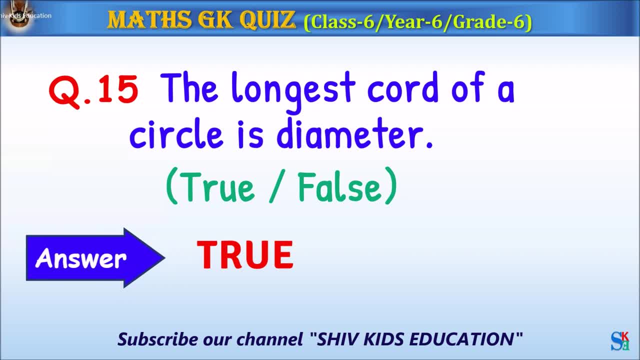 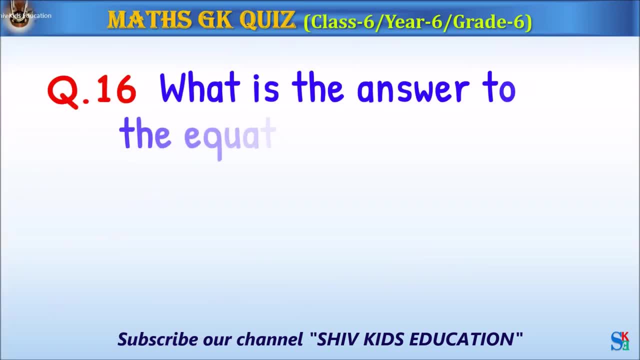 True or False? The answer is True 15.. The longest chord of a circle is diameter. True or False? The answer is False, 16.. What is the answer to the equation below? The answer is 0. 17.. What is the calculation below in standard? 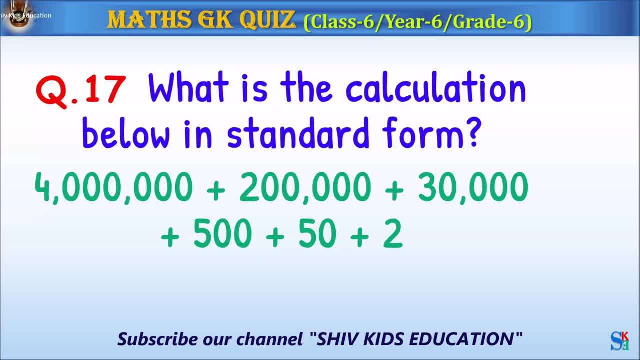 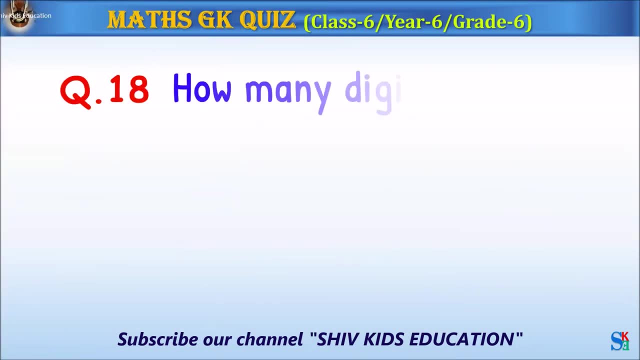 form? The answer is 4,002,000.. True or False? The answer is 2.30,552.. SAMC Sutra 2.. lucky numbers: 8.una has twoине kini 19.. How many pourquoi digits are there in 4,567?? 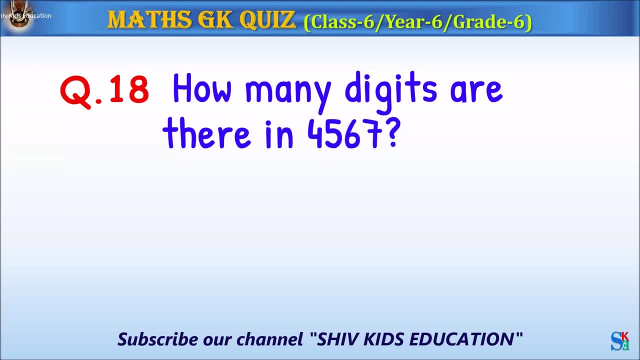 True or False? The answer is 4, 7.. How many digits are there in 4,567?? The answer is 4- 8. 19.. How many have unemployed people to notice? Believe it or not? 2.33,669?. Okay, Let's do a 4.. einfach, 4, 3.11, 7.1, 9.ñaí'viete en tuyado'nya, La respuesta es 4, 7.11, 7.11, 7.2, 7.du documents 3 e a 4: 224. 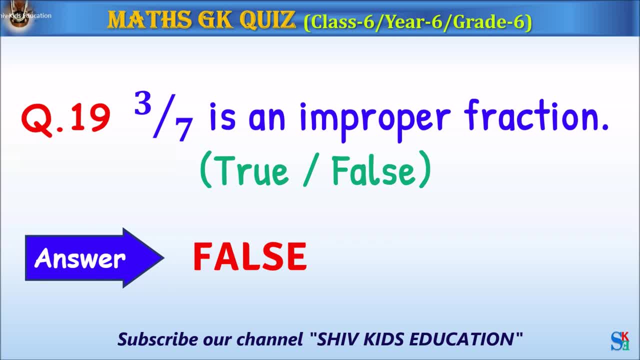 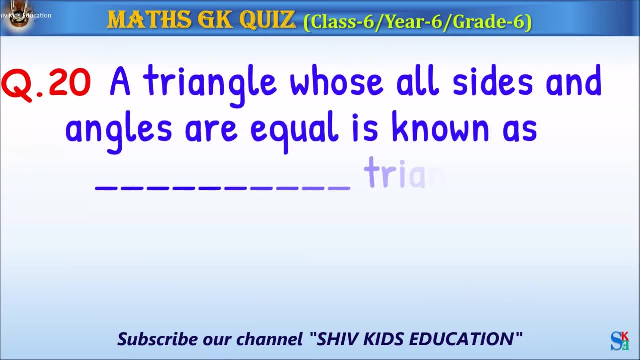 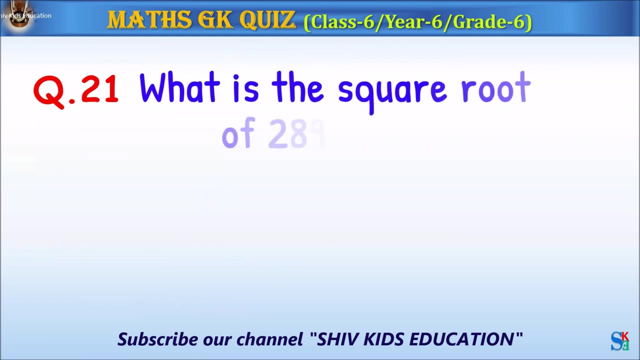 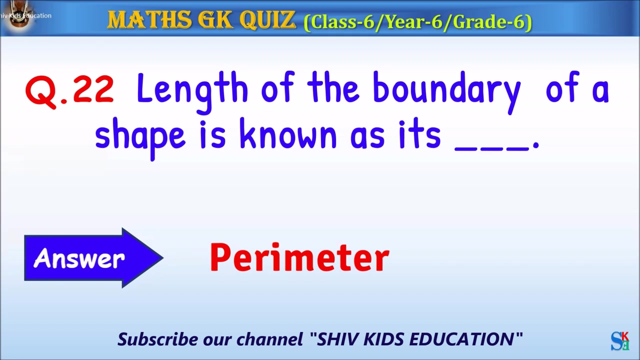 The answer is False. 20.. A triangle whose all sides and angles are equal is known as what triangle? The answer is Equilateral triangle 21.. What is the square root of 289?? The answer is 17: 22.. Length of the boundary of a shape is known as its what. 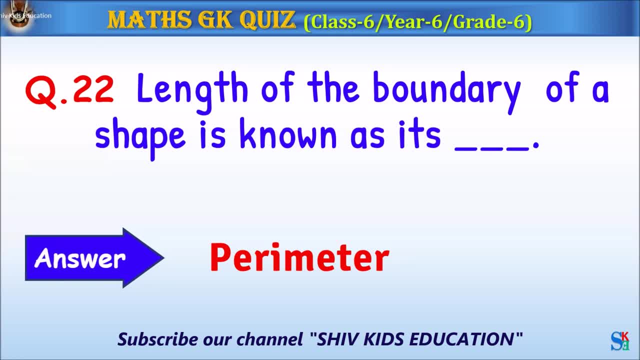 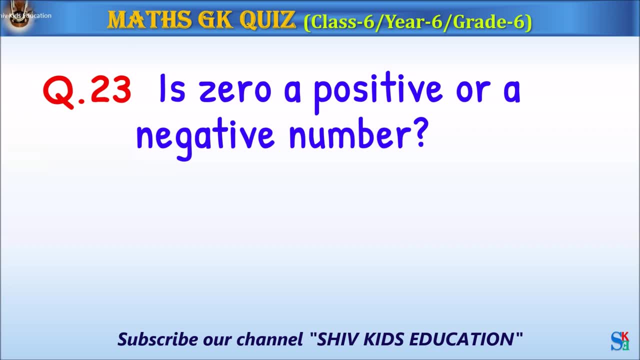 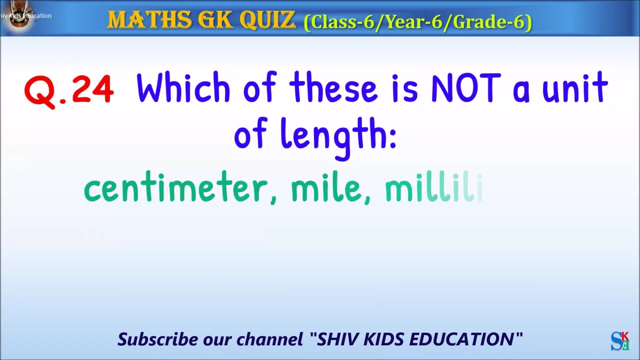 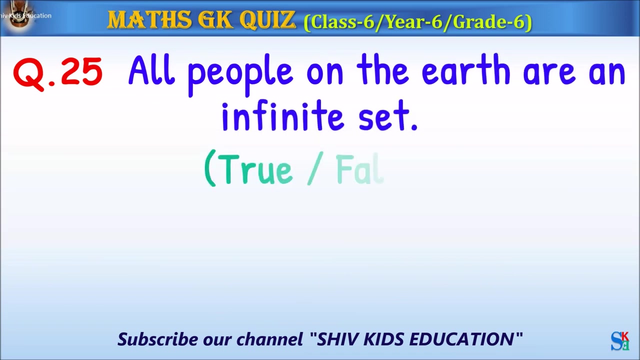 The answer is Perimeter 23.. Is zero a positive or negative number? The answer is None of the two mentioned above 24. Which of these is not a unit of length? The answer is Milliliter 25. All people on the earth are an infinite set. 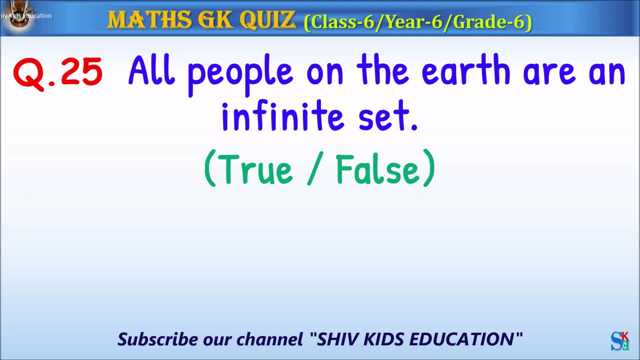 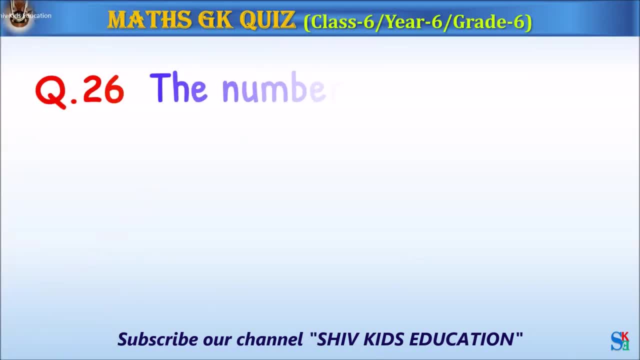 The answer is Milliliter 25.. All people on the earth are an infinite set. The answer is Milliliter 25.. All people on the earth are an infinite set, True or False? The answer is False 26.. The numbers which are not multiples of 2 are known as what? 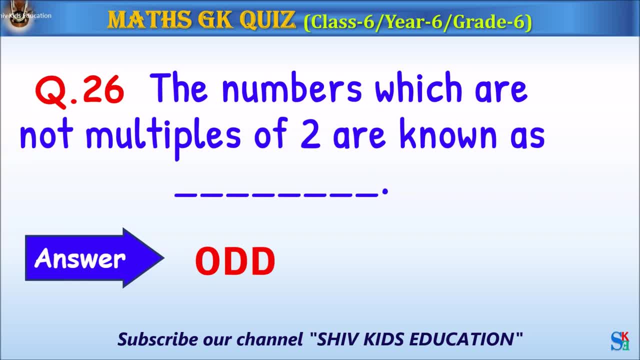 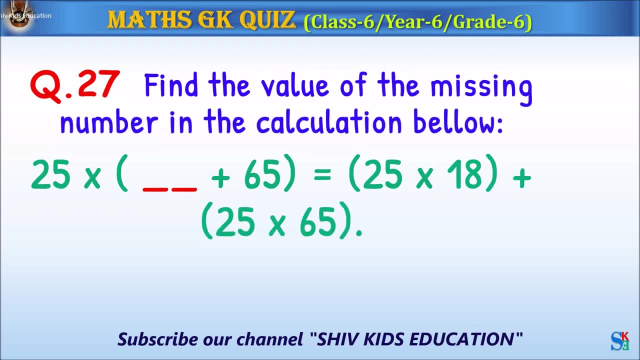 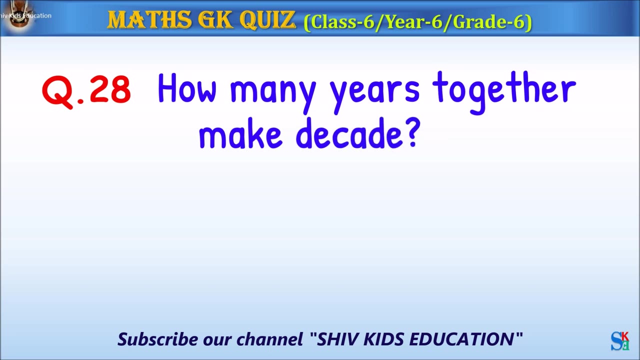 The answer is Odd 27.. Find the value of the missing number in the calculation below. The answer is 18. The answer is 18. 28. How many years together make a decade? The answer is 10. The answer is 10.. 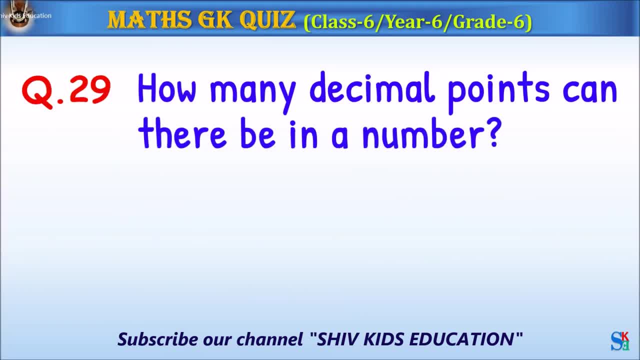 29. How many decimal points can there be in a number? The answer is 10.. The number obtained in a chapter is semblingly even, but you have to put in the prove rules. The answer is 2. The answer is 2.. 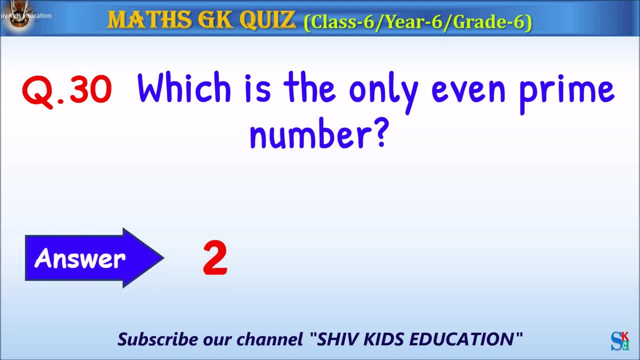 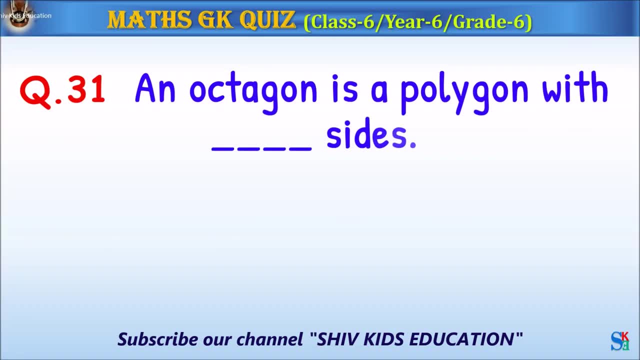 So the answer is 17.. Now let us donc on the math and impart the answer 30, which is the only even prime number, The answer is 1.. The answer is 2.. Thanks, Branch 31.. An octagon is a polygon. with how many sides? 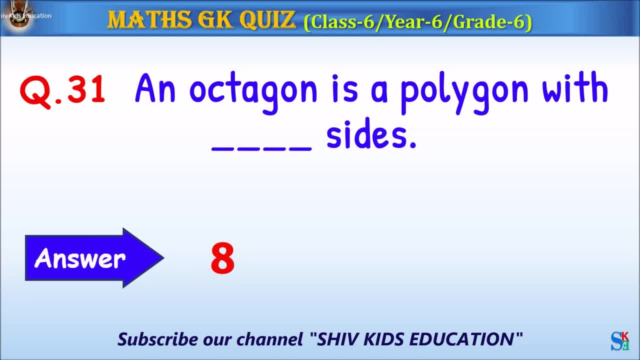 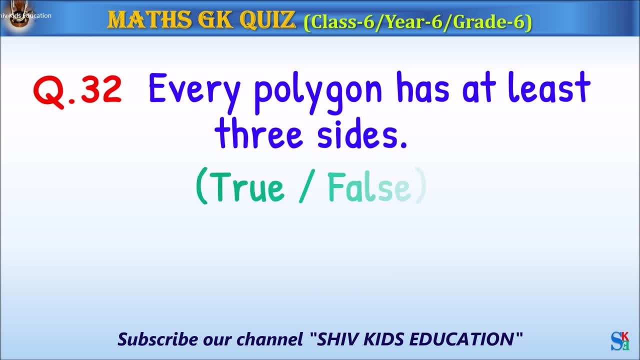 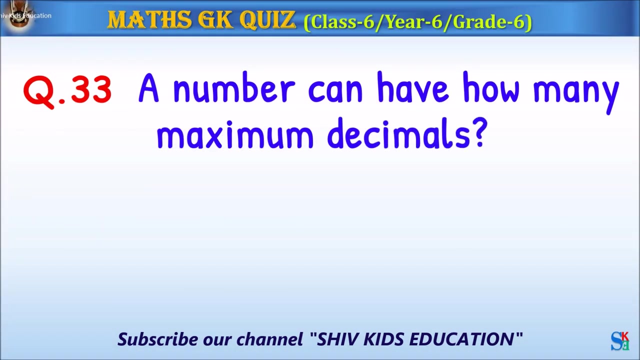 The answer is 8.. The answer is 2.. The number mentioned above is constantly changing, 32. Every polygon has at least three sides, True or False. The answer is True, 33. A number can have how many maximum decimals. 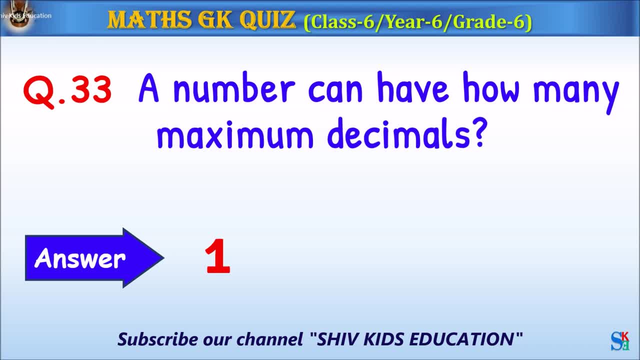 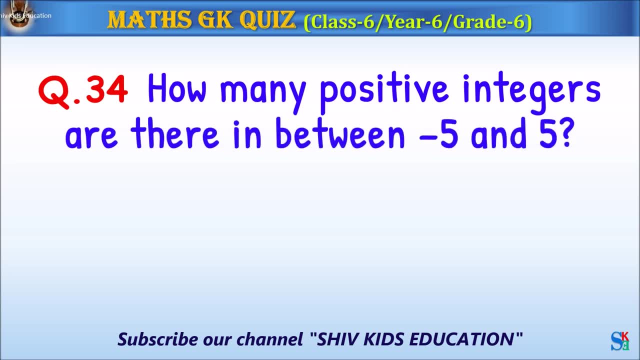 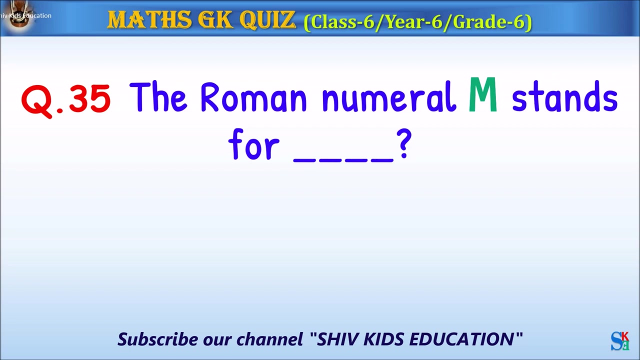 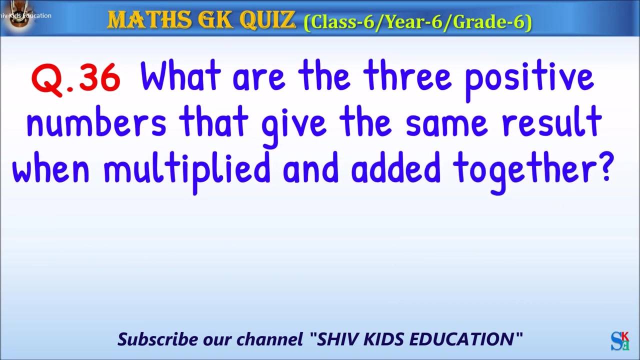 The answer is 1. 34. How many positive integers are there in between minus 5 and 5?? The answer is 4. 35. The Roman numeral M stands for what? The answer is 1000. 36. What are the three positive numbers that give the same result when multiplied and added? 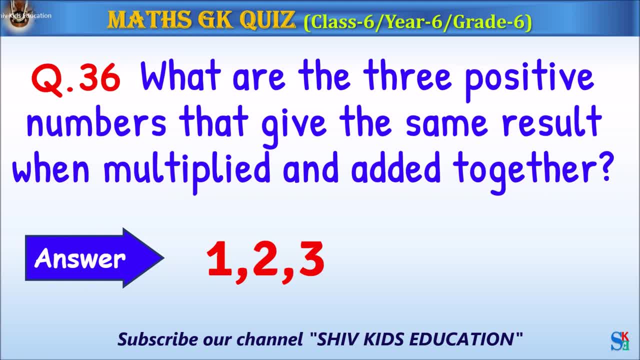 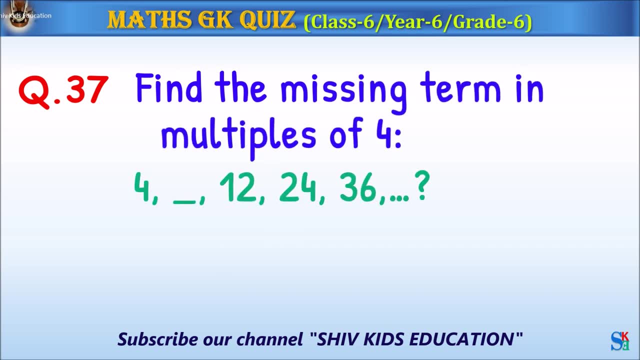 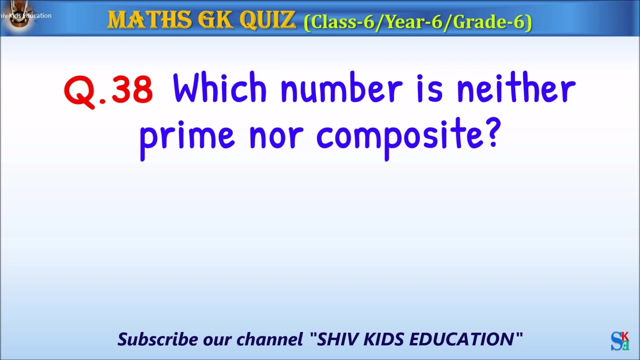 together. The answer is 1, 2 and 3.. 37. Find the missing term in the multiples of 4.. The answer is 8.. 38. Which number is neither prime nor composite? The answer is 1.. 39. An angle whose measurement lies between: 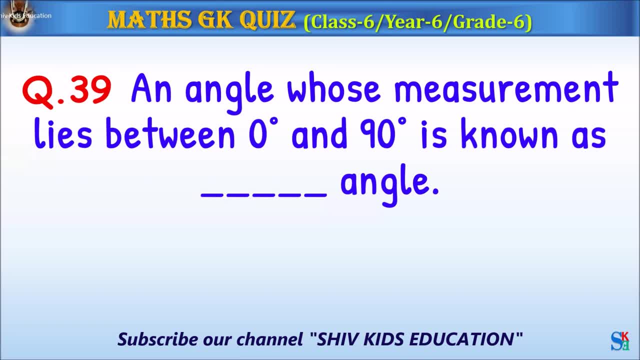 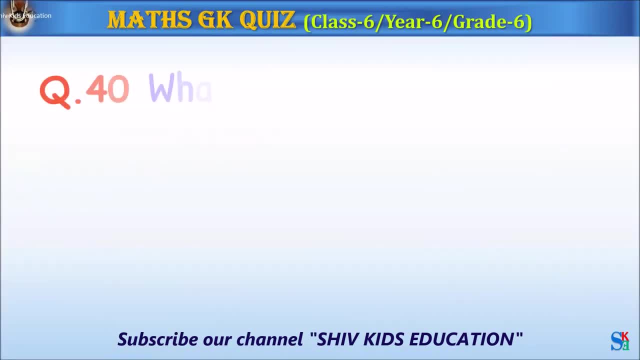 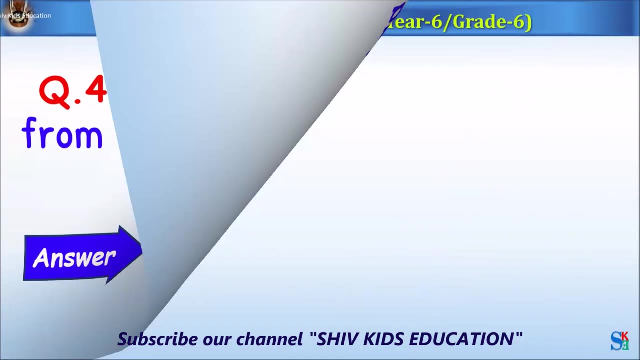 0 and 90 degrees. is known as what angle? The answer is Acute 40.. What is the value of A from the below given equation? The answer is 4.. 41. 0 divided by 567 equals what? 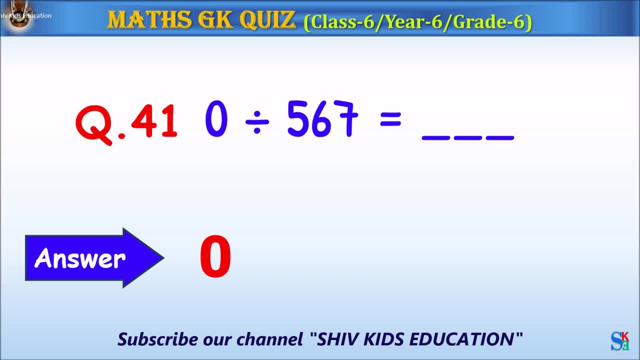 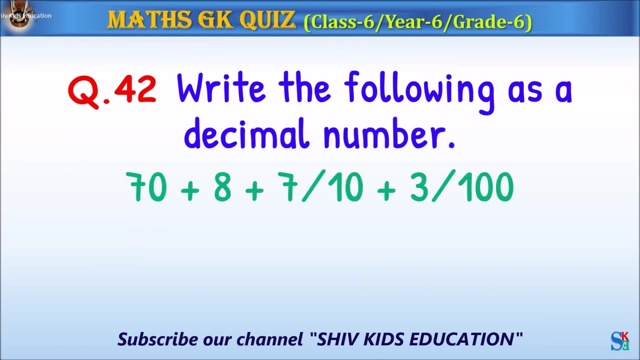 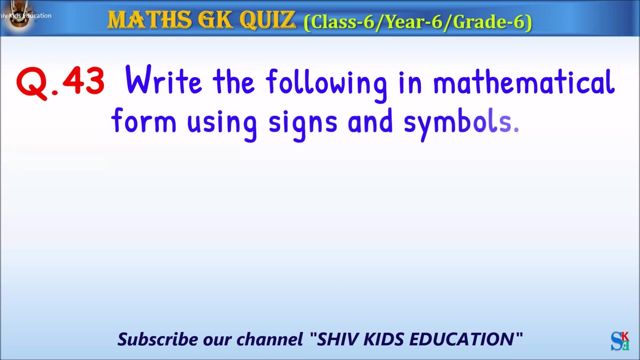 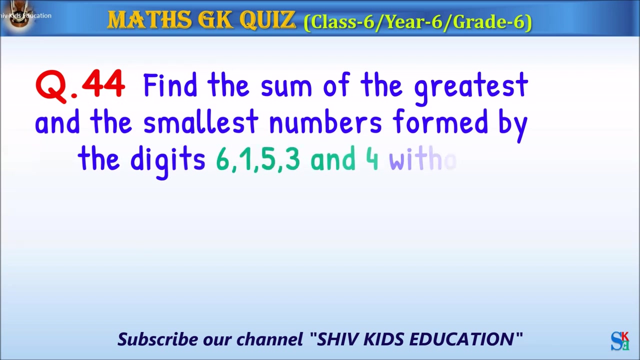 The answer is 0.. 42.. Write the following as a decimal number: The answer is 78.73.. 43. Write the following in mathematical form using signs and symbols: The answer is 64.. 64.. Find the sum of the greatest and smallest numbers formed by the digits 6, 1,, 5, 3 and 4, without repeating any digit.